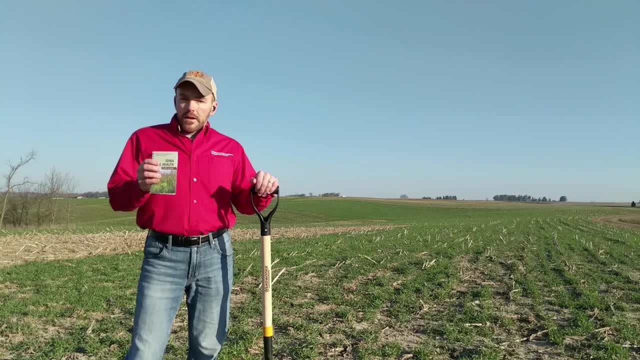 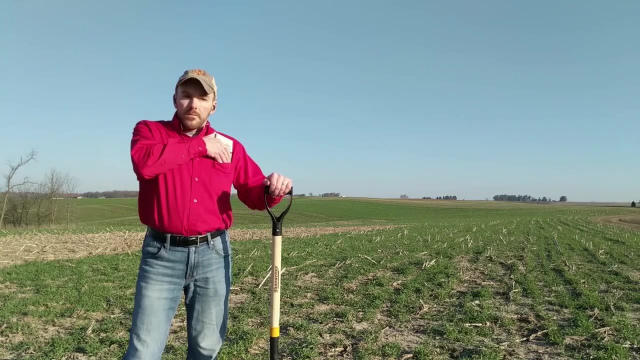 This is available through the extension store. But in this guide there's a little assessment card in the back that you can use to score your soil health. So that's one option. You can just Google soil health assessments. You might be able to find some. 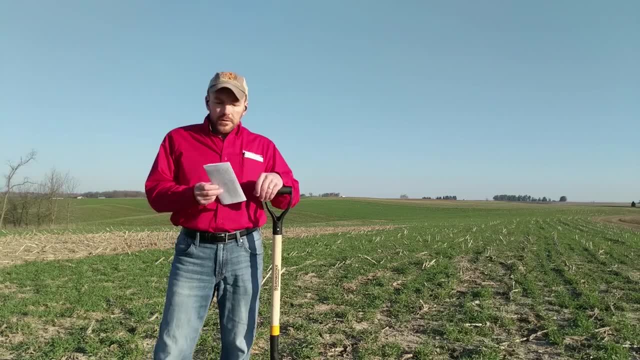 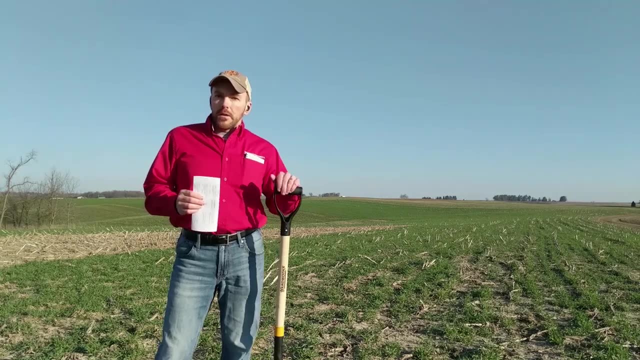 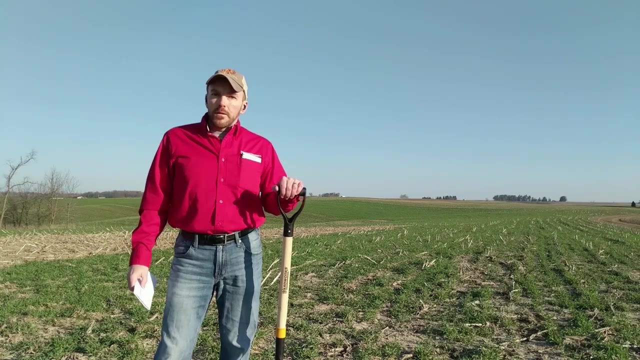 others online. I've also got one here that I put together. It's just kind of a combination of a few different assessments. I'll post my contact information at the end of the video with my email, So you can feel free to call me or shoot me an email and I'm happy to give you a copy of this. 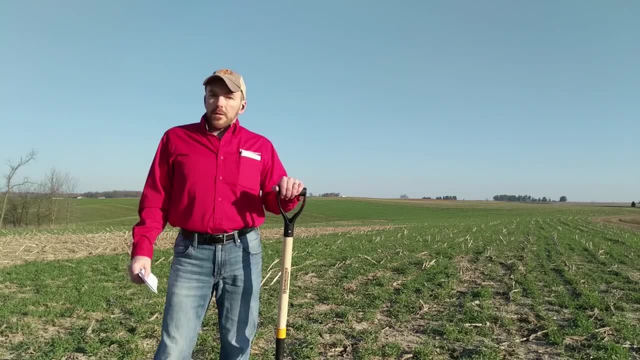 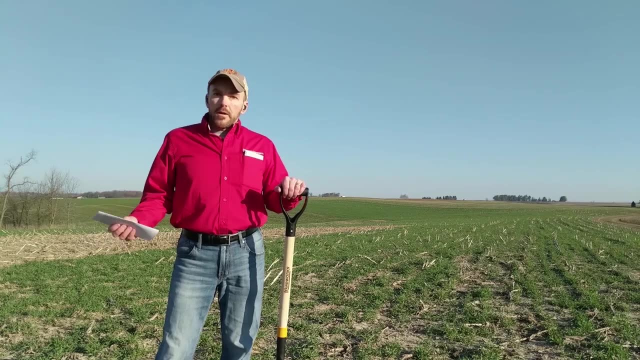 free of charge. So another good thing to have is a camera Just take pictures, Just some way to keep a record of what you've seen. So that way if you want to compare, you know one field to another, you've got a way to kind of assess that. You know these are somewhat subjective obviously. 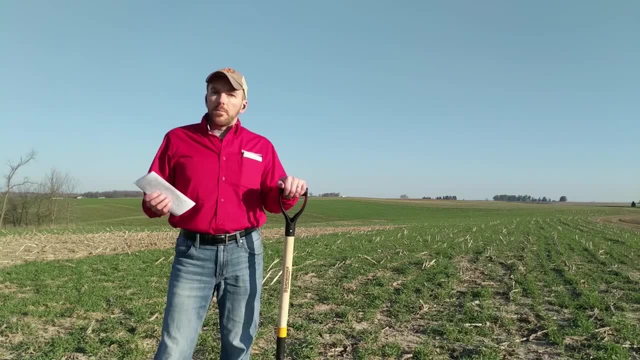 because you know every person will have a different idea of what the score should be. But at least if you're doing the assessment, you know you have a fairly reasonable way to track. that. That's also great. if you want to track it over time, You know, come back to the same field two or three years. 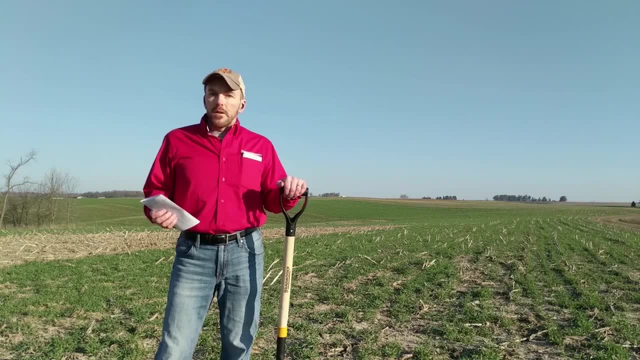 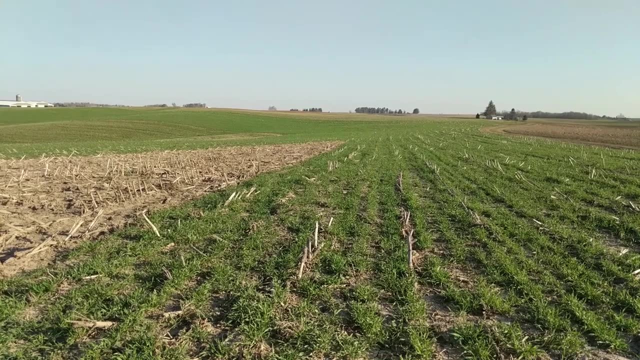 later you can see how your soil health is progressing. So let's dig some holes Before we start evaluating the soil. I want to give you a little bit of a background on the site here where I'm going to be pulling these samples. 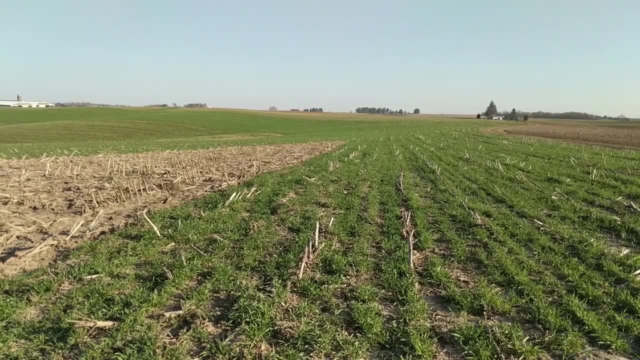 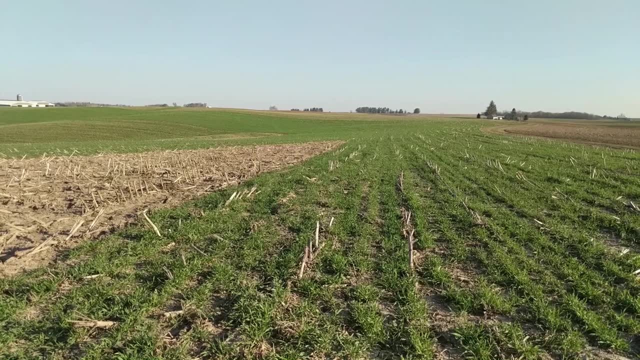 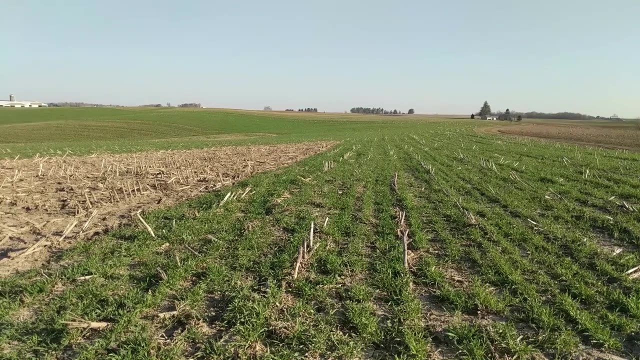 So this is actually a family farm up in Elm Key County here, So very northeastern Iowa. These are Fayette silt loam soils, And so what I'm going to do here, the field we're looking at was in corn last year, So it was corn silage was chopped off last fall. 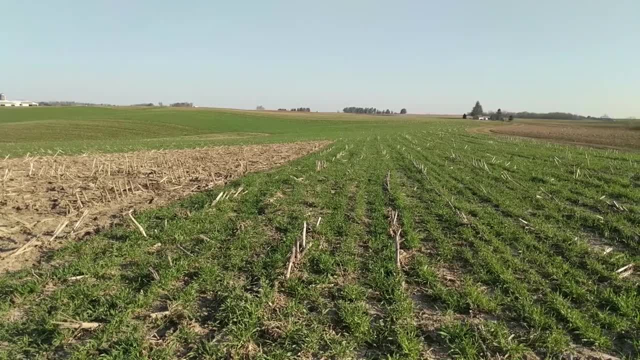 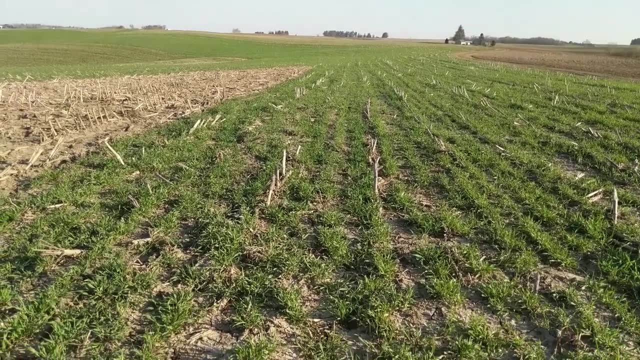 It had dairy manure applied, It was tilled and then seeded to a cereal rye. So this is the cover crop. So on the right here you see the cover crop. So what I'm going to do is pull up some soil from this cover crop here. 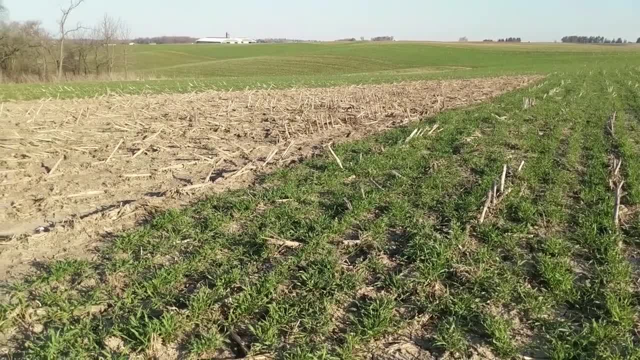 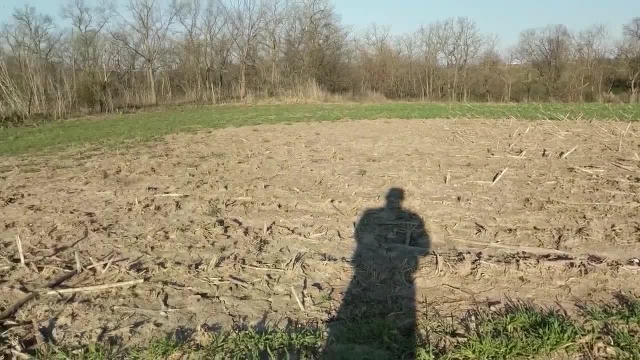 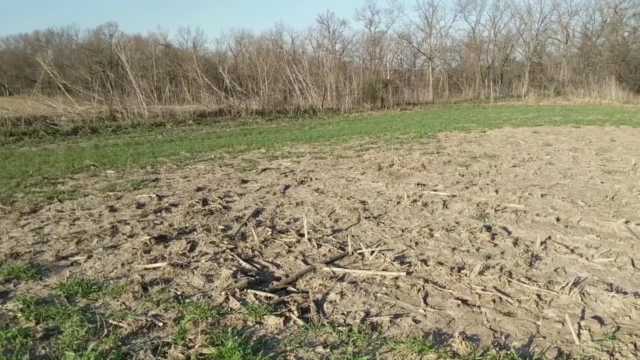 You can see some point rows here that were skipped, So I'll pull up some soil from that area. We can compare that to the cover crop ground, And then over here is an old fence line, And so this is a really good idea if you're doing a soil health assessment, to try to find some area nearby. 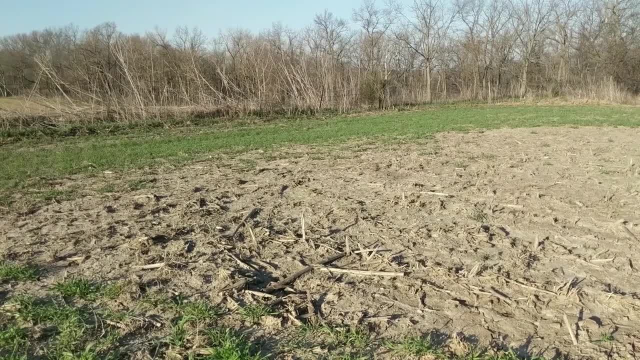 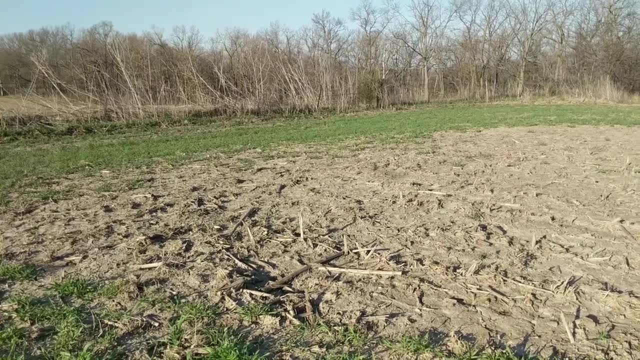 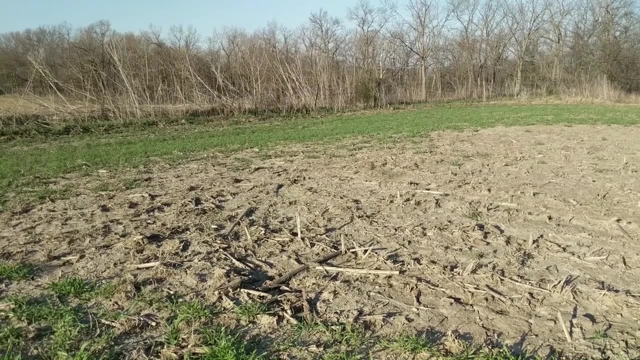 that's soil type that's been undisturbed- Ideally you've got some perennial vegetation on it- been undisturbed for a long time- And that kind of gives you a baseline to compare your soil to. So if you can find some soil somewhere nearby and that way you can kind of get an idea maybe what your soil used to look like, 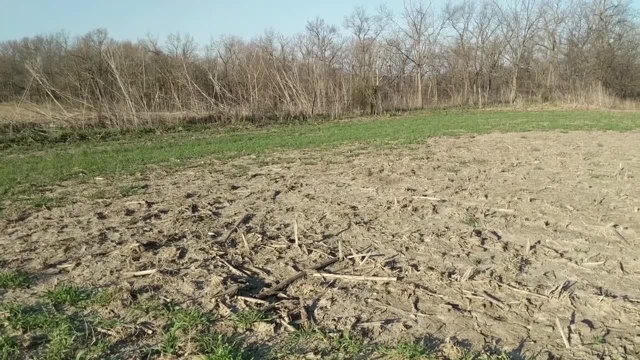 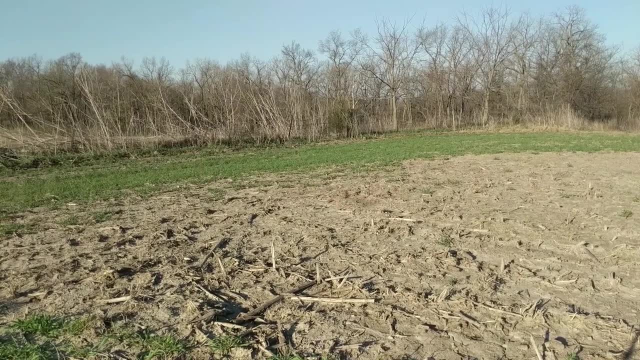 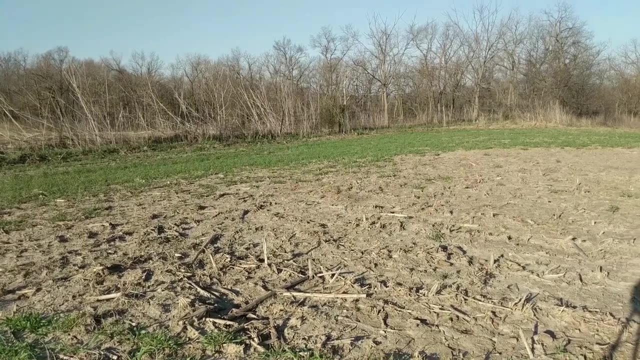 or what it potentially could look like if you start working on soil health. So I highly recommend that As a comparison and that kind of gives you a benchmark when you're doing your soil health scoring. So the first thing I do- doing an assessment before I would even dig up the soil- is: just take a look at the surface. 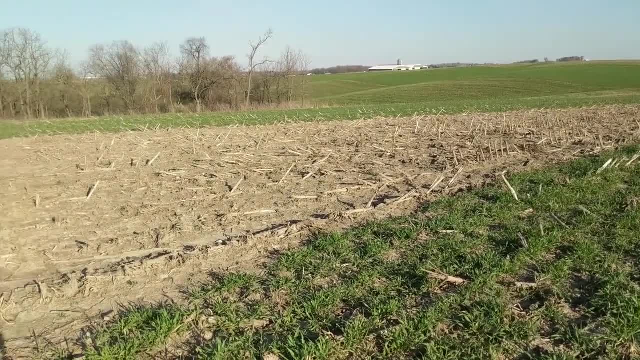 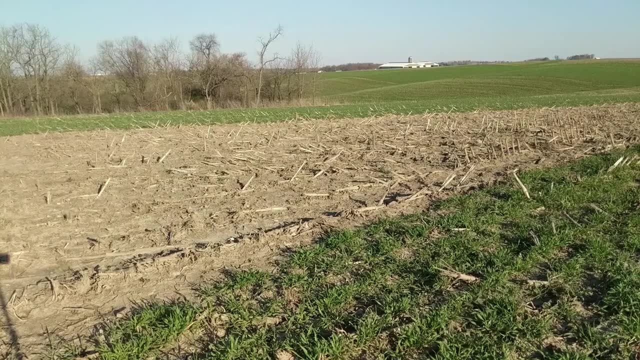 And so this ground here obviously quite bare. you know it had corn silage, so very little residue It was tilled up. There's basically no surface cover there, And so I would score. that you know pretty good. 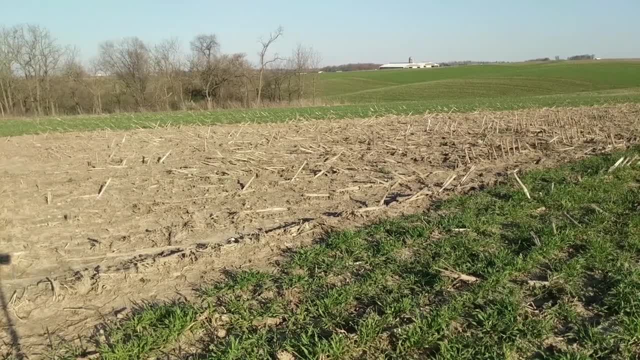 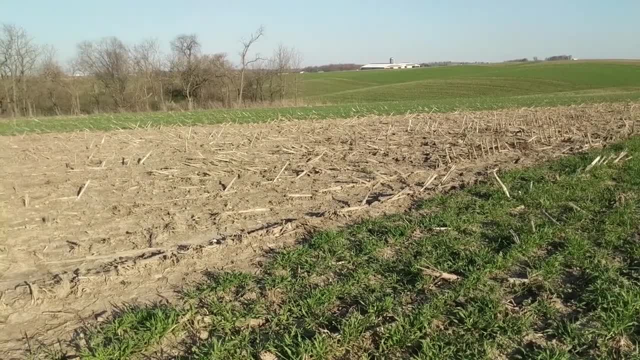 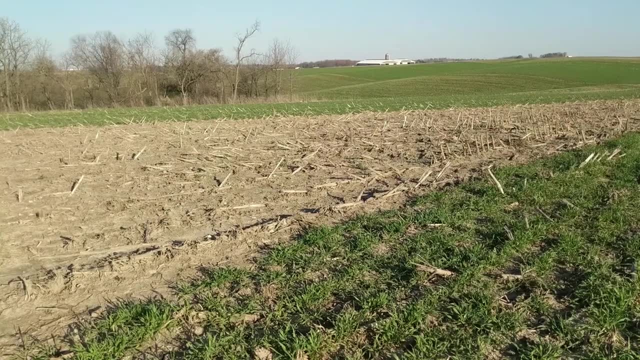 You know I'd probably give that maybe a 2, you know There's some evidence of surface crusting there, So just generally not in great condition based on surface cover. So come over here to our cover crop. you know definitely much better. 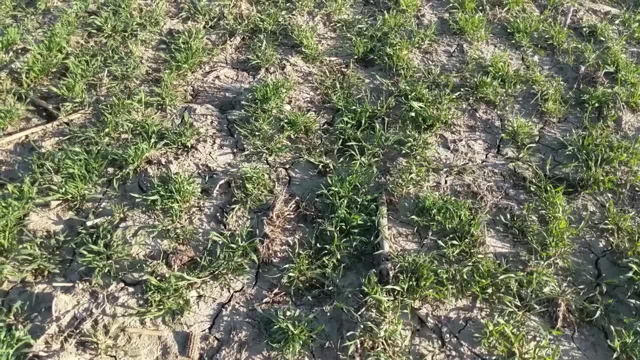 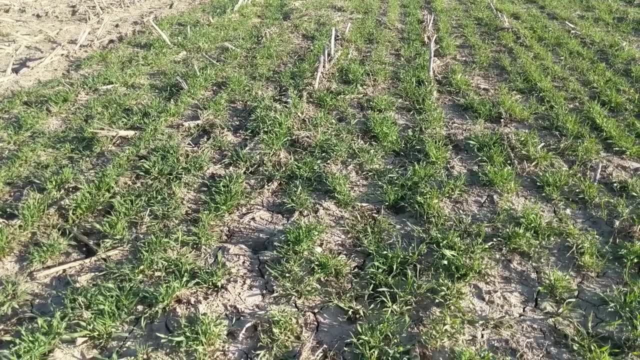 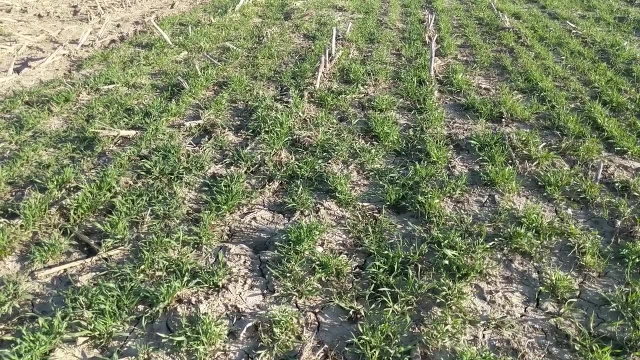 We've got some ground cover there, but still some bare spots. you know, not much residue in between. you know I'd maybe score this. you know maybe a five. So again, very subjective, but once you do a few of these you'll get the hang of it. So now I'm going to dig up some soil from these three. 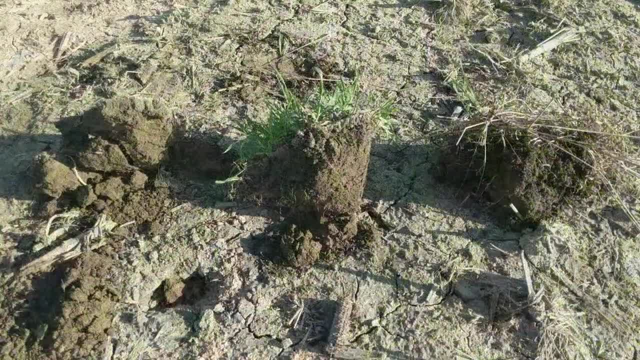 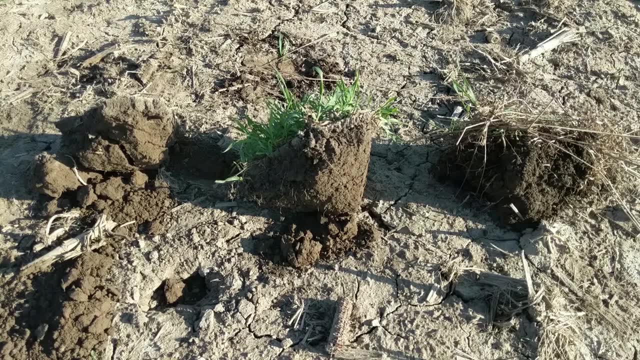 areas and we'll take a look. Okay, we've got our three samples pulled up here, So what you're looking at on the left is a sample from the bare ground here, where the silage is chopped off. The one in the center is from the cereal rye cover crop And the one on the right is from 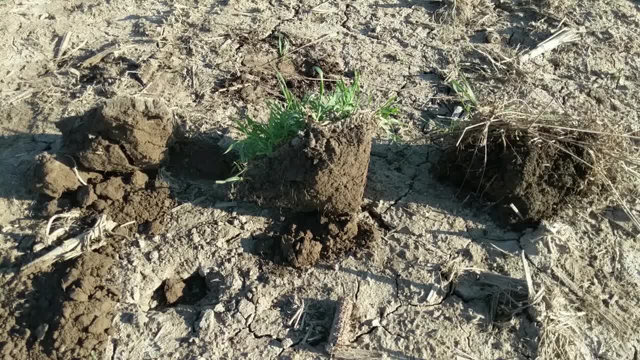 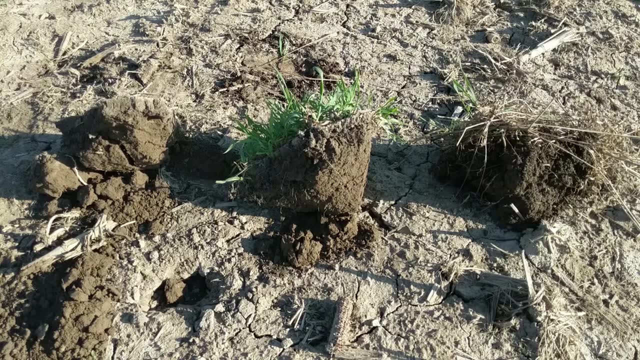 the fence line. So one of the first things you would look at doing a visual assessment is color. So I hope you can see this on the camera here. but you can clearly see that that soil from the fence line is a darker color than the other two. So good indication there that there's probably 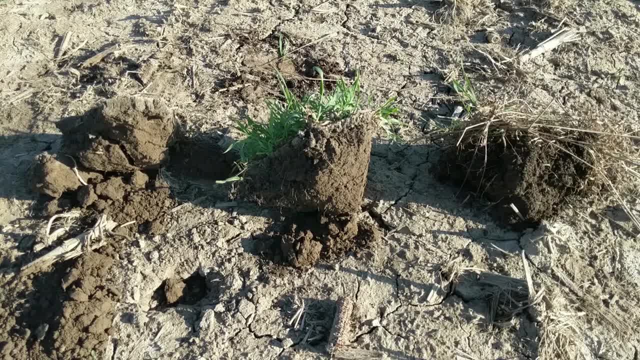 quite a bit more organic matter in that soil, So you have to be a little bit careful, you know, when you're assessing color, because it will change depending on the moisture content of the soil. So just make sure you're doing an apples to apples. 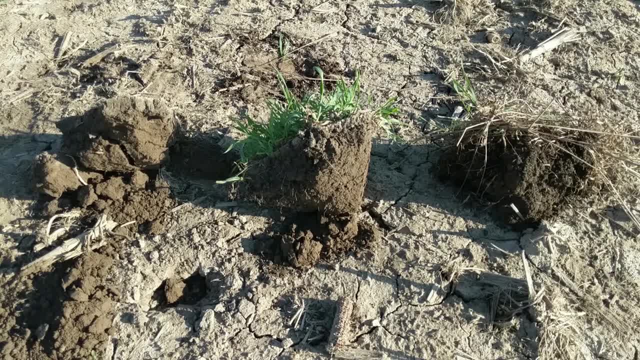 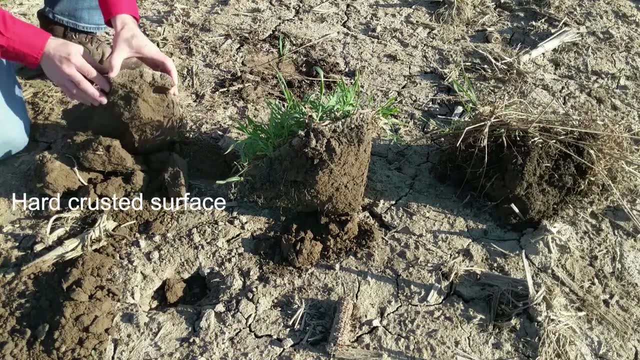 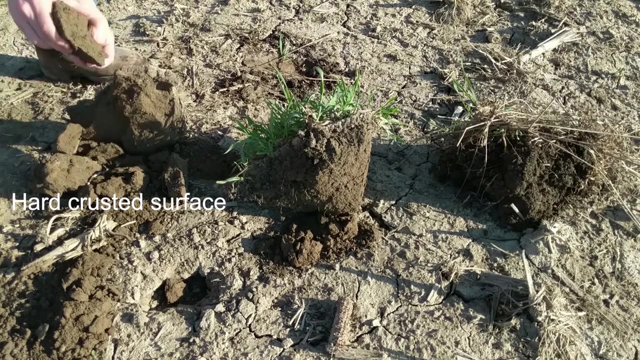 comparison there. So the second thing I would start looking at would be: you know kind of the structure of the soil or the aggregation of the soil, And so you can see on the left here, where we had our bare ground, The soil is very- I'd call that- platey. There's not a lot of structure there. 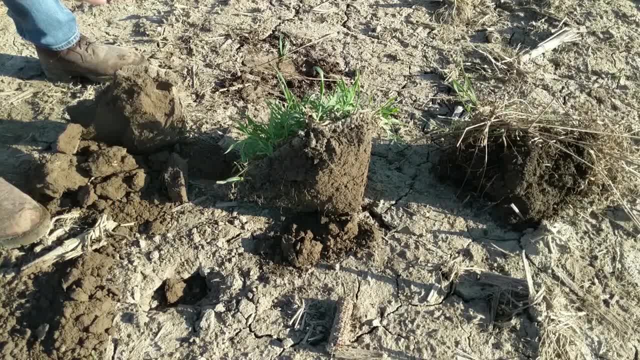 You break this open. it's just, it's pretty homogenous because of the tillage. There's some micro aggregates there, But, you know not, it crumbles fairly easily, So that's a good sign, But you know. 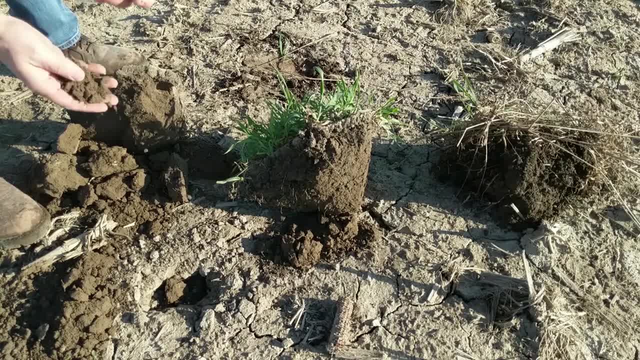 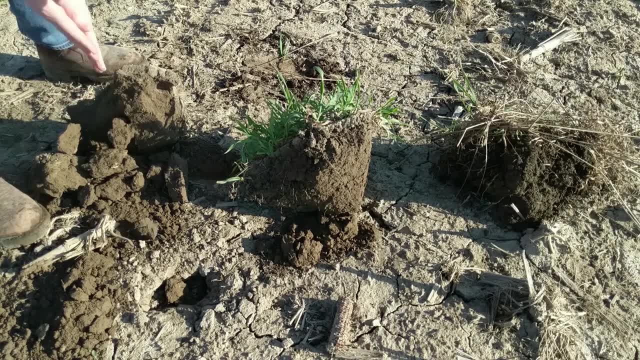 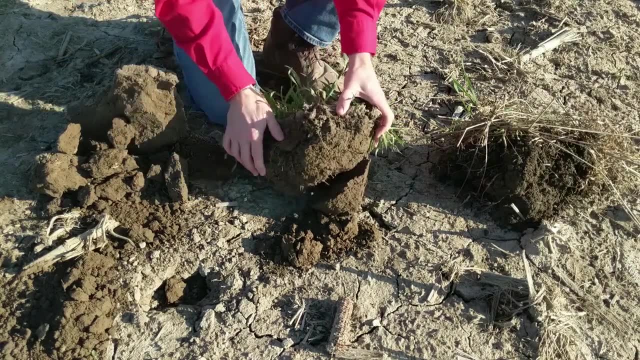 not a lot of good aggregation there because we don't have any roots growing here And so that's kind of preventing this soil From aggregating. So now we look at our cereal rye cover crop. So what's kind of amazing to me is, you know, these were both tilled. 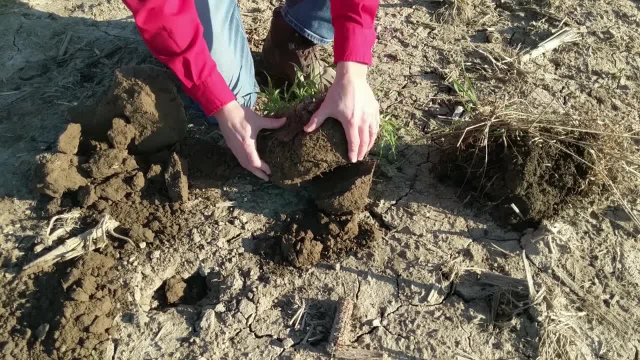 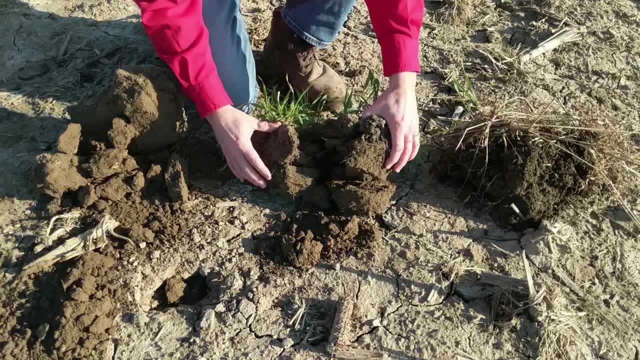 last fall. But if you look at this cover crop you know we've only got a couple inches of growth here on the surface. But look at the aggregation. It's already starting here Just within a few months with this cover crop. 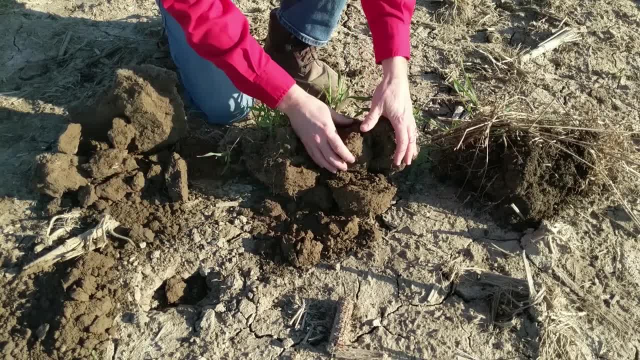 we've got roots down Probably almost a foot. I didn't dig all the way down, But you know. so this can be a little misleading. You know, you might look at a cover crop. it doesn't look like there's much there. 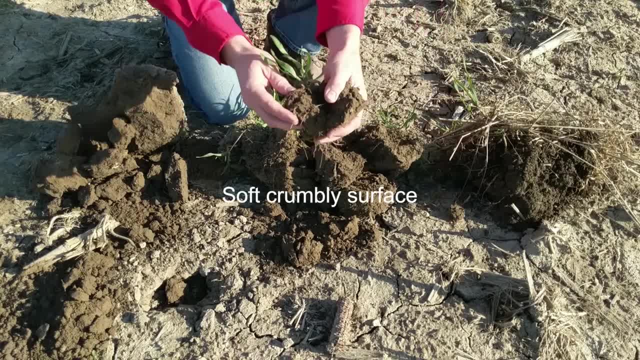 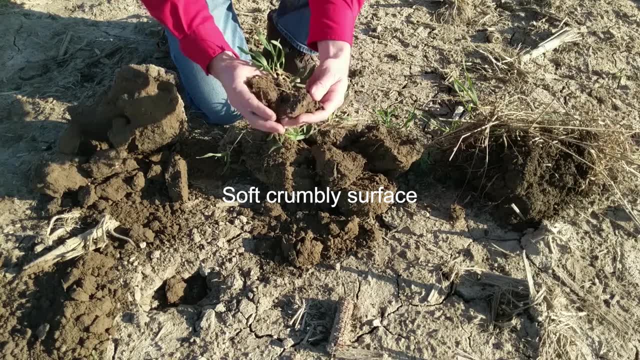 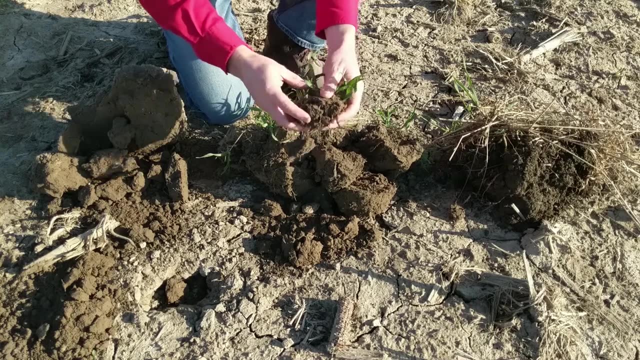 But there's a lot more going on below ground than above ground. We've got earthworms in here. You know this soil is going to hold together much better in a rainfall event. You know these roots really help hold it together. You can see the aggregation starting there, So